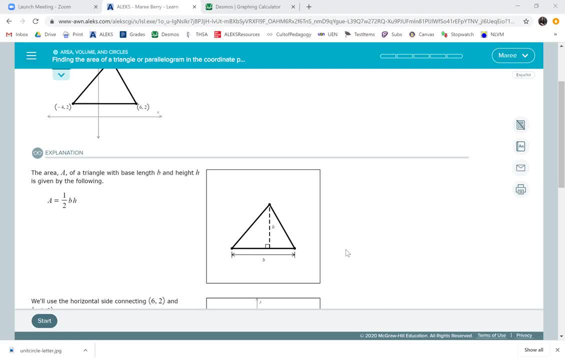 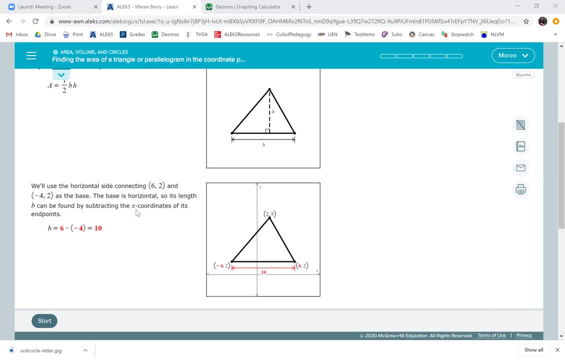 So you have to make sure that the base and height are perpendicular on both triangles and parallelograms. With a triangle, we have to remember to divide by two after we multiply base times height. So, um, to find the, the, how far apart they are, you can take the x values and subtract them. So six minus a negative, four is a positive 10.. So this is 10 apart. 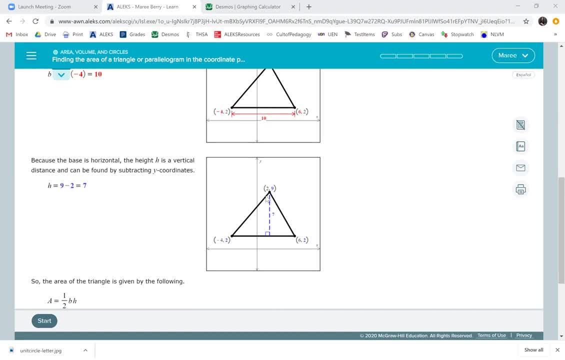 Or if you count the spaces, that will help too, And then the Um to see the height, you see how far apart the y's are. So nine minus two is seven, So you have 10 times seven, and then divide it by two and you get 35.. So we'll do some examples, We'll have some parallelograms. Good, So the distance between 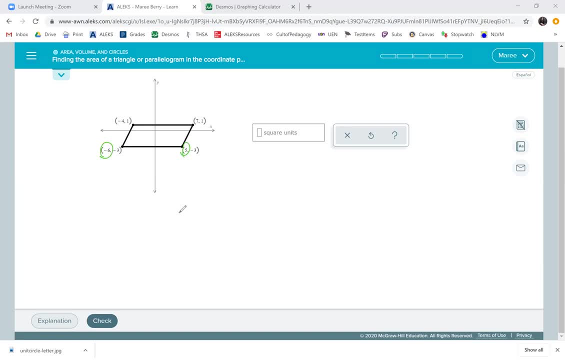 The bases is five minus a negative six, Which is 11.. So the base is 11.. The height is- We're going to do the y, So one minus a negative three, Which is four. So the height is just straight up and down, which is four. So for parallelogram we just do base times height. So this is 44 square units. 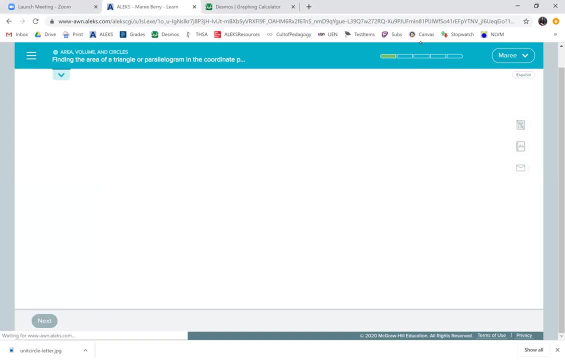 Okay, we'll do next one. This triangle is turned on its side, so Don't let that stress you out. We're still. we want to know the distance here. So this one's the y value, so negative one minus A negative seven. It's kind of like seven minus one, which is six, and then the height. We're going to go the distance between the x's, so negative five minus. 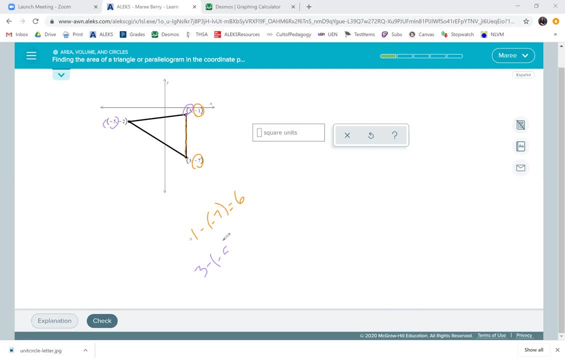 I mean three minus negative five. Sorry, If you were to do negative five minus three, you get a negative eight And you just do the absolute value of that, because distance can't be negative. So this is a positive eight. So because it's a triangle, We want to do six times eight and then divide by two. So that is 24.